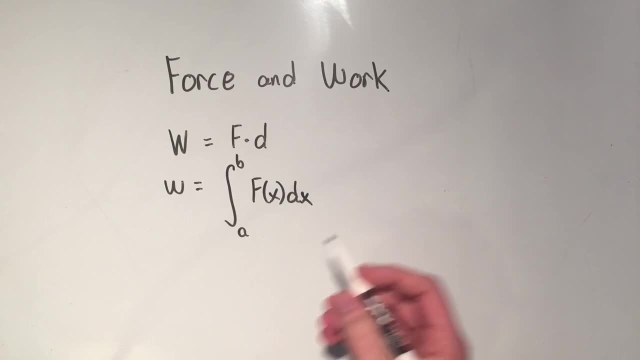 So I have a pretty easy problem here. Let's just say that your force function is the line 3x minus one, And you're going to do that from one to five. So you can imagine yourself pushing a block along this path for one to five. you could think of it like that, Or? 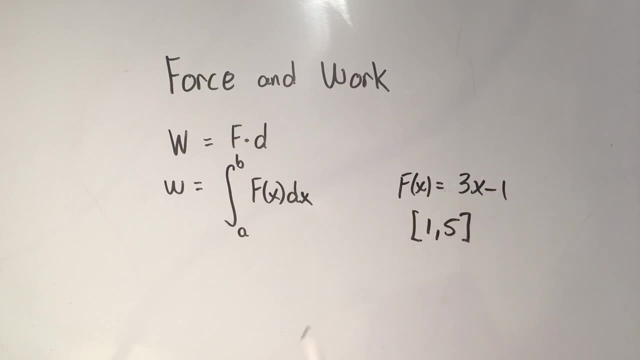 you could just think of. this is the amount of force and you got to integrate it over that interval. So we're just going to do that really simple, definite integral from one to five And I'm integrating 3x minus one dx. And now, if I take the antiderivative of this, 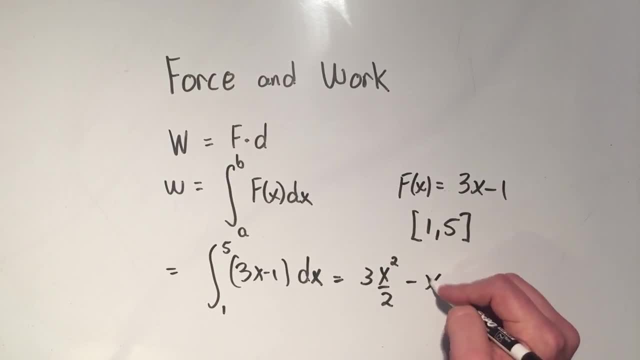 add one to the power divided by the new power, the antiderivative of minus one is minus x, and I have to evaluate from five to one or one to five, And I just plug in the upper limit, plug in five minus, plug in the lower limit, plug in one, And now I can evaluate this thing. So let's see. 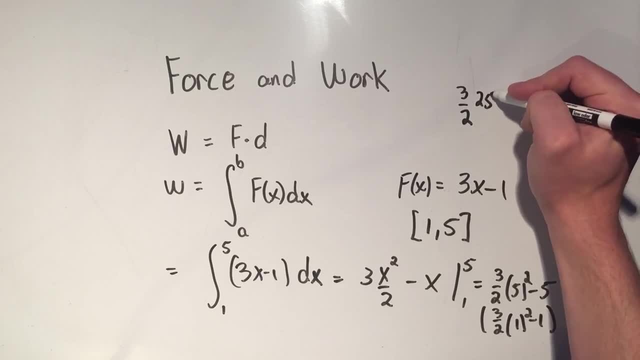 that's three halves Five squared is 25, minus five minus one squared is one. So that's minus three halves And I have minus minus one is plus one. And let's see, I've got minus five plus one. Let's see it's going to. 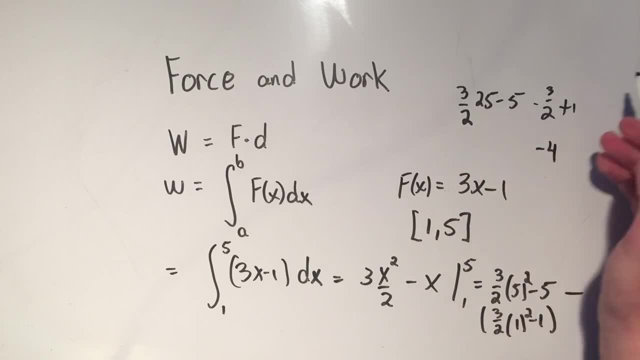 be minus 425 times three is 75 halves Minus three halves, And then 75 halves minus three halves at 72 halves minus four and four is eight halves. So 72 minus eight- I think that's going to be 64 over two- is 32.. So the amount of 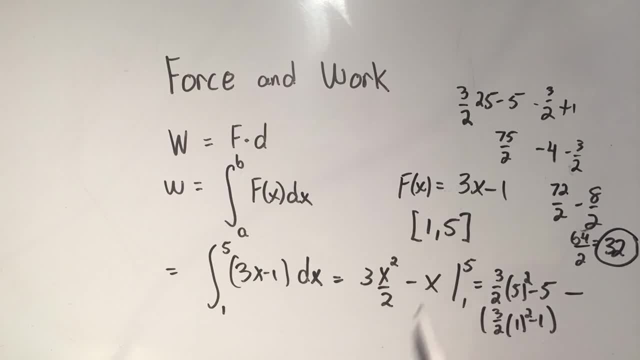 work that you've done by using this force function over this interval is 32 amounts of work. So, whatever units you're using with. Okay, there's your quick introduction to force and work. you just got to remember that you do the definite integral from A to B of your force function. Thanks for watching.